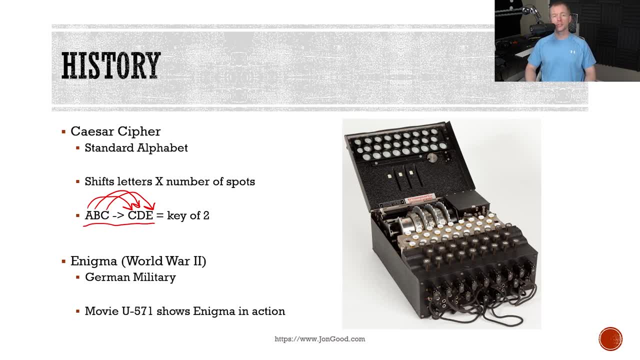 Then we write our message by using the shifted letters. During World War II, the German military used a device called the Enigma in order to encrypt their messages. There's actually a movie that was made in the year 2000 about capturing one of these devices, and it was. 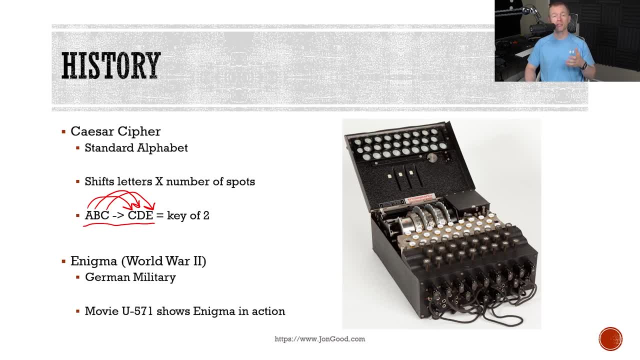 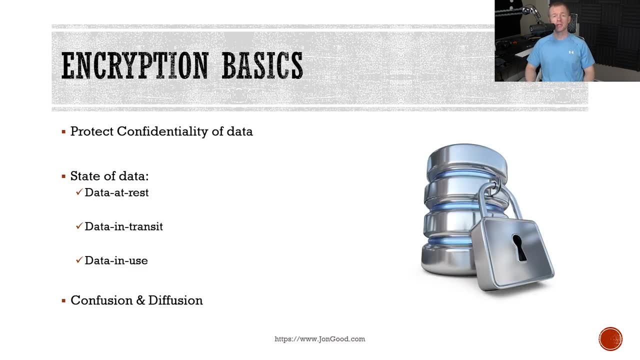 called U571 with Matthew McConaughey. Today, you can actually find the Enigma machines at World War II museums. The biggest reason for using encryption is to protect confidentiality. Remember that confidentiality is the concept of keeping secrets a secret and preventing unauthorized people from actually seeing that data. When we talk about encryption, we might 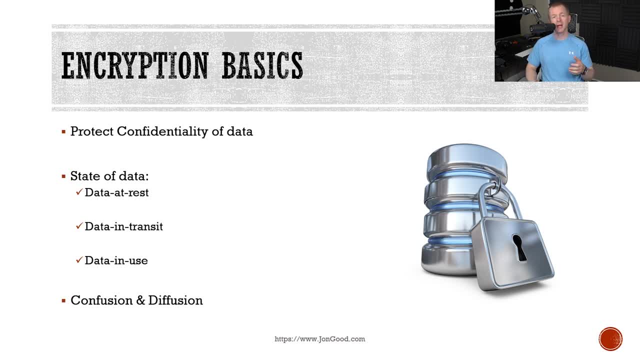 also reference the actual status of the data. We have data at rest, and this is when data is actually sitting on a hard drive or in a database somewhere. We have data in transit, and this is when data is moving across the network between two different systems, For example. 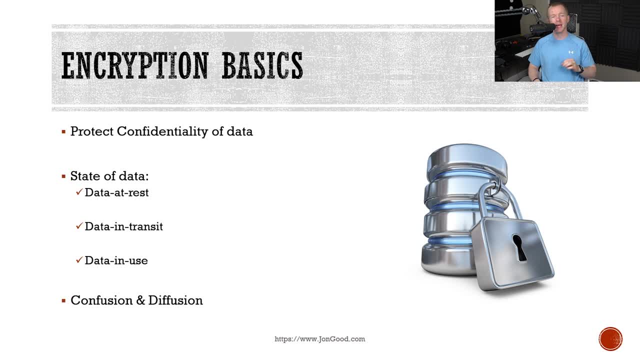 we might have a client that's browsing the web using HTTPS and all that traffic is encrypted, And then we have data in use which refers to when a system is actually using that data. So, for instance, if a system can't use that data in its encrypted format, it will unencrypt that. 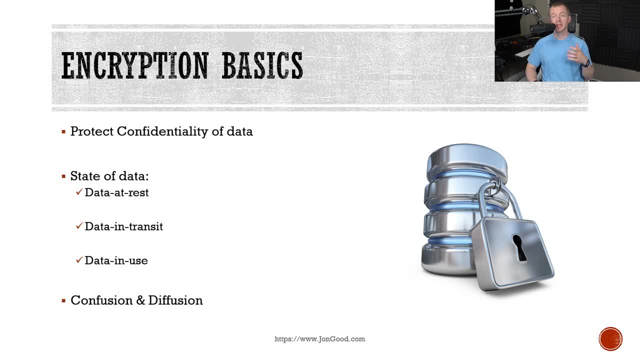 data and it will store it in memory while it's using it, And this is really common with things like applications, especially so like a database or something like that. We also have confusion and diffusion, which are important concepts for encryption. Confusion means that the ciphertext 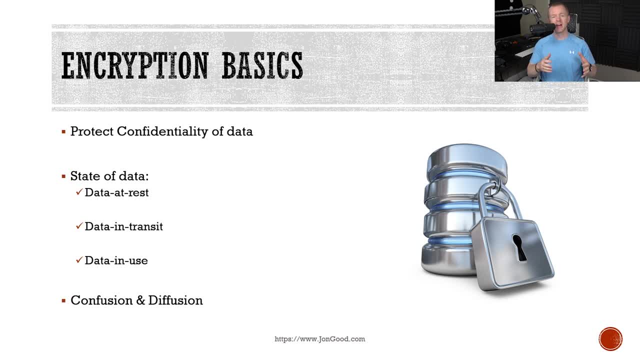 that encryption algorithms create actually is very different than the actual plain text. So, for example, if we have our plain text as just hello, so just the word hello, then with confusion this might actually be something completely different, So you cannot get hello. 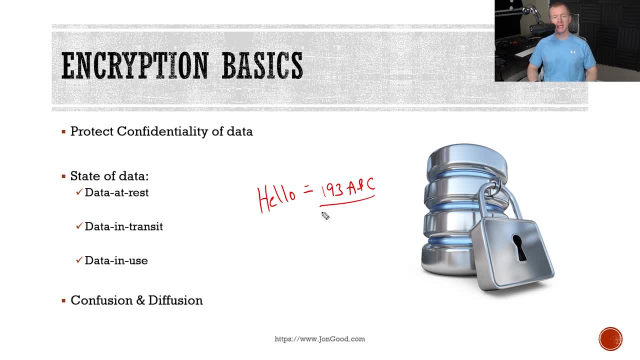 out of that. And then diffusion is where small changes in the plain text create major changes in the ciphertext. That way, if one character is changed, the string is going to be completely different. So that way, using our same example here, if instead of hello we have hello, 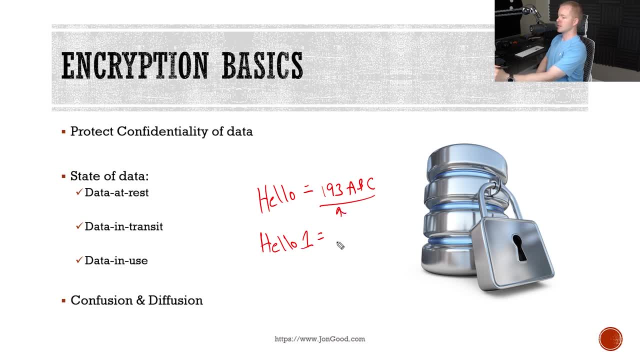 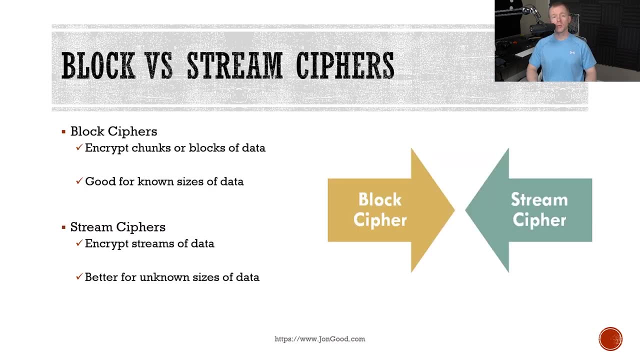 one, then maybe, instead of this string here, we actually get something completely different. When we talk about encryption, we also have to be aware of how the data itself is encrypted. There's two different ciphers that you need to be aware of when it comes to encryption. 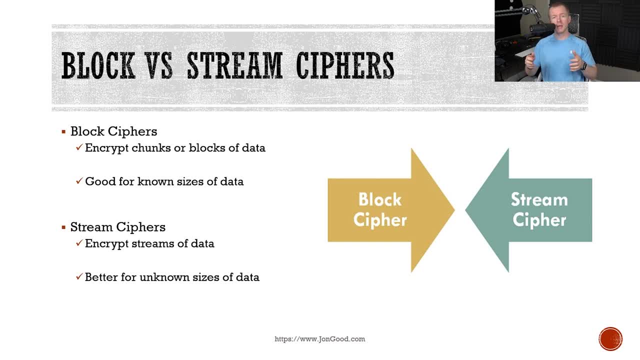 First, we have block ciphers that encrypt data in chunks Or blocks, such as 64-bit or 128-bit. This is great when you actually know the size of the data. We then have stream ciphers, which encrypt data in streams of bits or bytes, and can actually be. 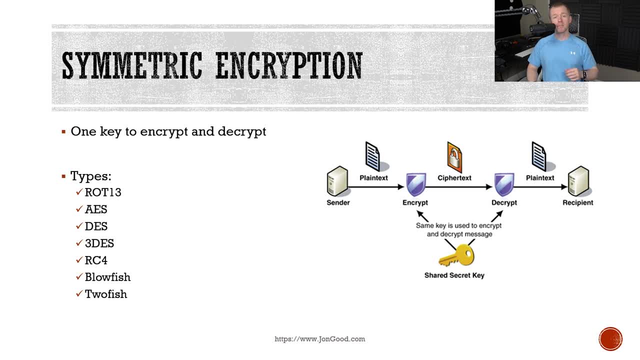 really good if we don't know the size of the data. Now we're going to get into the main types of encryption. We're first going to start out with symmetric encryption and then we'll move on to asymmetric encryption. With symmetric encryption, we're using the same key or a pre-shared key. 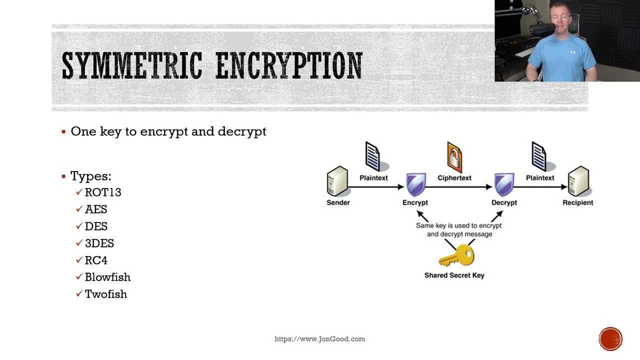 in order to decrypt and encrypt the data. That means that if you have that one key, you can do both encryption and decryption. One issue with symmetric encryption is that we can't necessarily verify who the sender or receiver is, because you're using the same key. 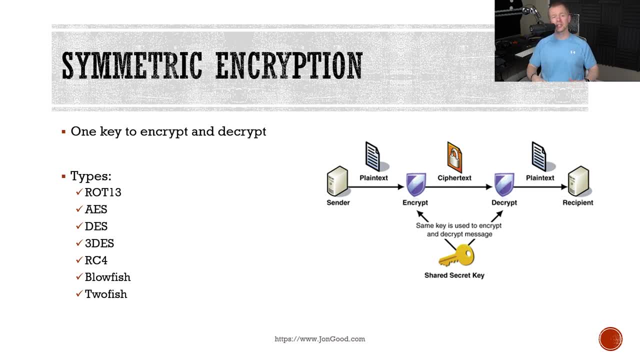 Another issue is how do we actually exchange that key initially. If that one key is intercepted, the whole process is no longer secure. I've listed some common types of symmetric encryption algorithms on the slide here. The most frequent that you might see are ROT13, AES, DES and triple DES, or three DES. 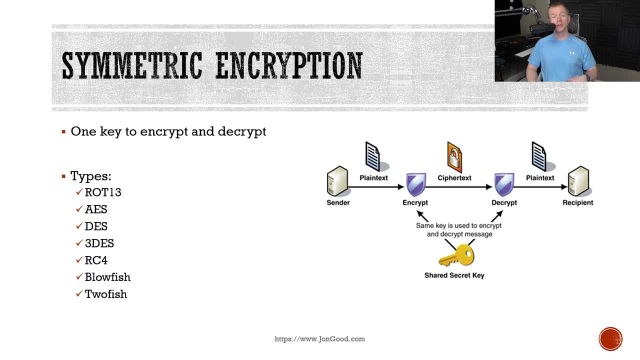 ROT13, AES, DES and triple DES, or three DES. ROT13 stands for rotate 13, and, going back to our Caesar cipher discussion, you would be rotating the alphabet 13 places. AES, or advanced encryption standard, is a very strong symmetric block cipher encryption standard. AES uses key sizes of 128,, 192, or 256 bits. 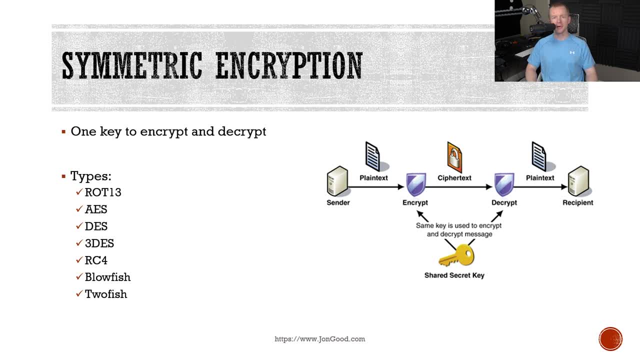 DES, or data encryption standard, is a block cipher encryption standard that encrypts data in 64-bit blocks, Triple DES or three DES. very similarly actually just runs that algorithm three times, So it's a little bit stronger than just normal DES, but it's still not stronger than AES. 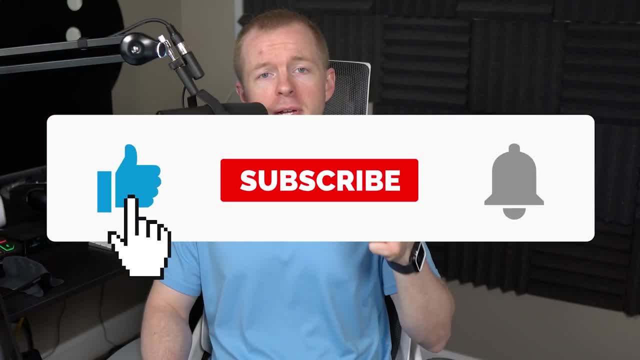 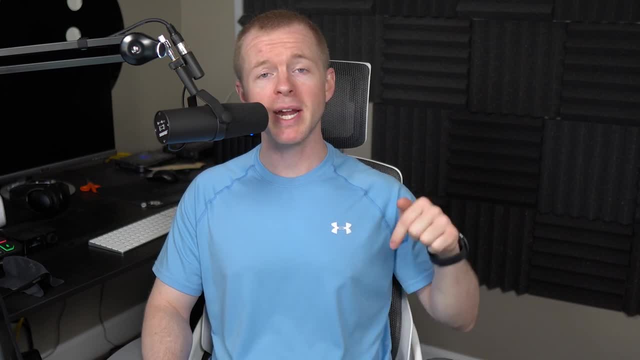 I hope that you're enjoying the content in this video so far. If you are, make sure to hit that thumbs up to like this video And if you think of any questions, let me know down in the comments section below. Also, remember that this training and courses can be found on my website at: 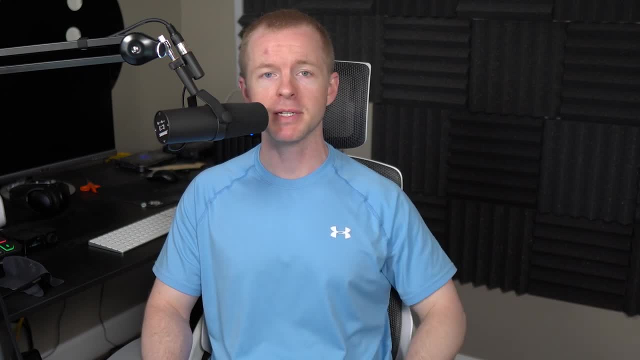 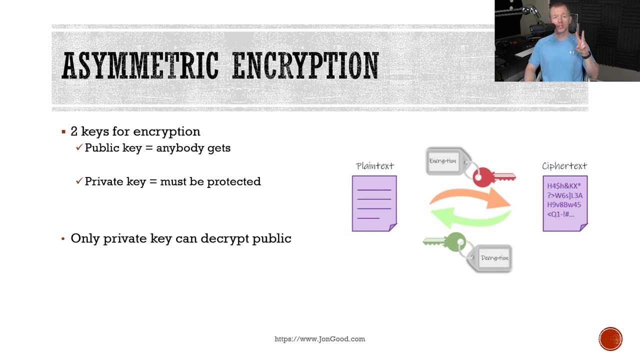 johngoodcom without distracting, interruptions or advertisements. All right, let's get back to the content. The second main type of encryption is asymmetric encryption. Asymmetric encryption uses two different keys, a public key and a private key, in order to encrypt and decrypt data. This is 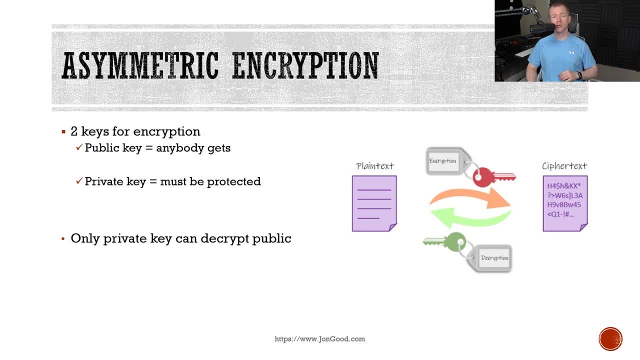 different than symmetric encryption because, if you remember, symmetric encryption uses the same key, so that one key for both encryption and decryption. Let's go over two different examples just to help you understand a little bit better. So in our first example, Alice wants to send an 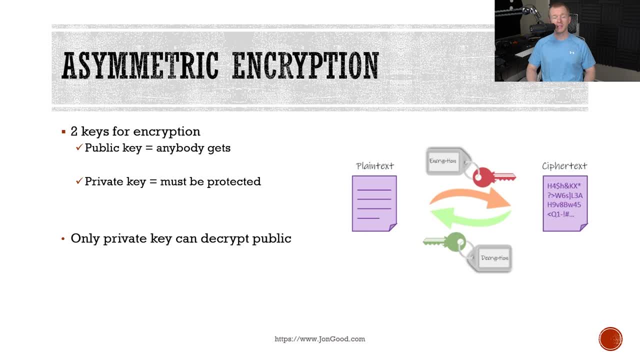 email to Bob, So she uses Bob's public key to encrypt the email. Bob then receives the email and he decrypts that email with his private key. In this example we can't necessarily validate that Alice is who actually sent that email, because Bob's public key 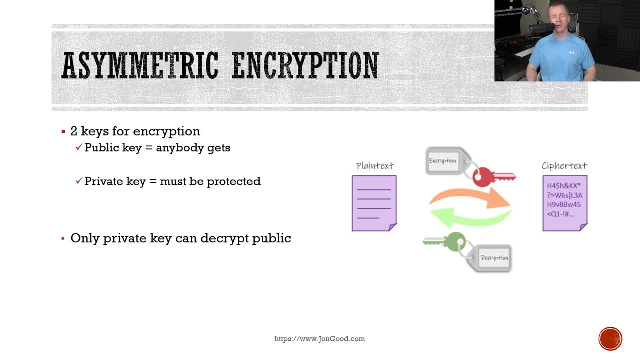 is actually available to a lot of people, but we know that it was unaltered because Bob was able to use his private key and decrypt that email. In our second example, Bob encrypts an email with his private key and he sends it to Alice. Alice then uses Bob's public key to decrypt the 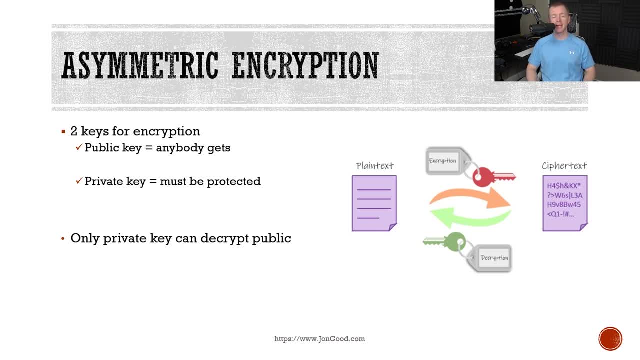 email. In the second example, we know that Bob actually is who sent that email, because he used his private key to encrypt that email. And then Alice used Bob's public key in order to decrypt the email In asymmetric encryption- one of the most important concepts- 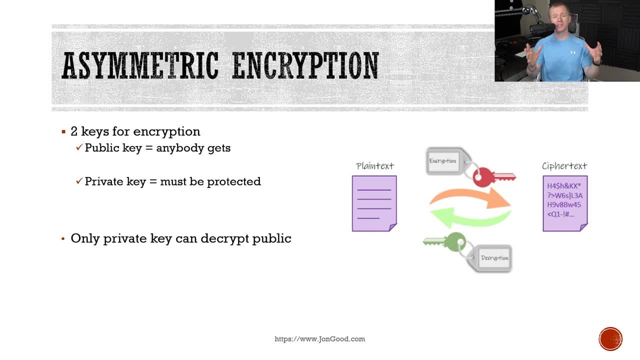 is protecting that private key because the entire system relies on that legitimate user being the only person that has that private key. If somebody intercepts that private key again, the whole system is not secure anymore. Question of the day, Since one of the issues with symmetric encryption- 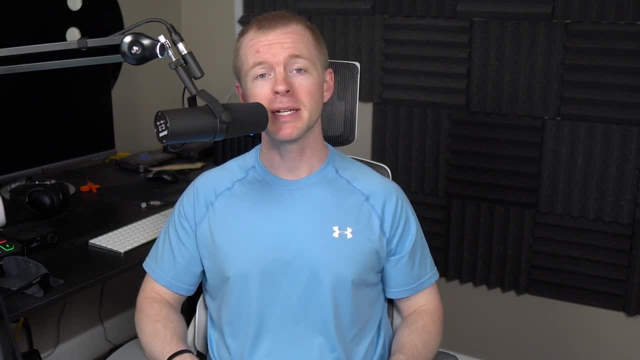 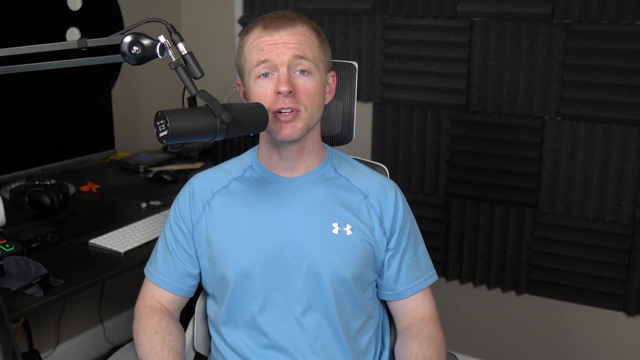 is that key exchange? what are some ways that we can implement in order to protect that exchange? I want you to do a little bit of research and let me know down in the comment section below. In this video we went over some history of encryption. 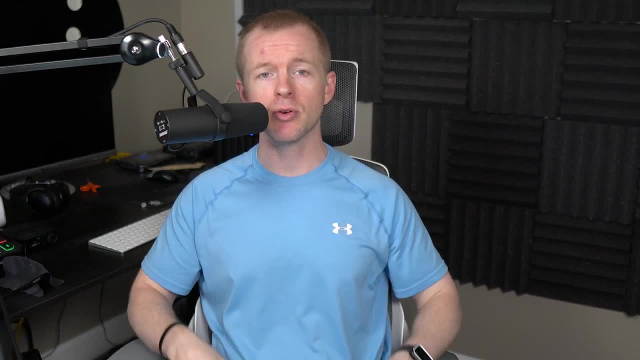 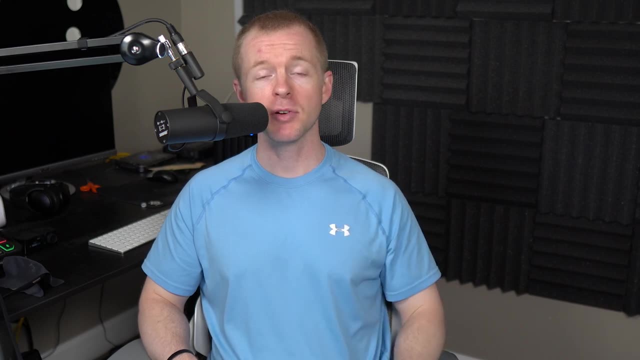 and then we broke down both symmetric and asymmetric encryption. Remember that with symmetric encryption, we're using a single key for both encryption and decryption, versus asymmetric encryption, which has a public and a private key pair. As always, make sure to like, comment and subscribe. 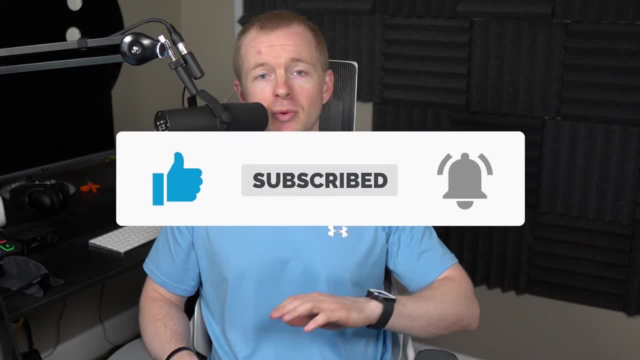 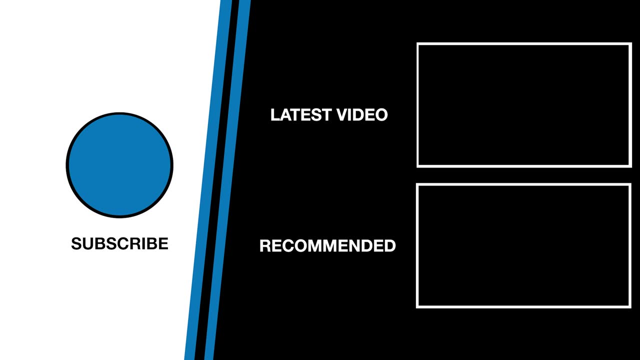 Check out my website at johngoodcom for more training without distracting, interruptions or advertisements, and I'll see you next time. Thank you for watching.